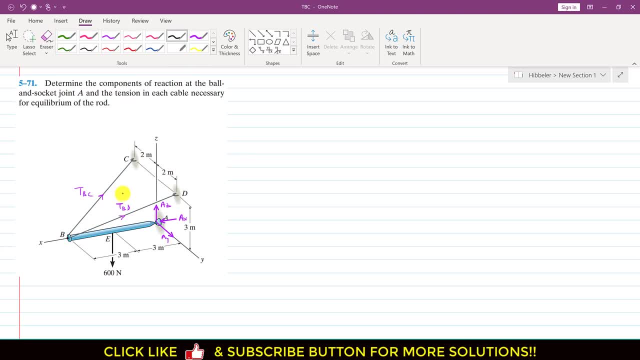 what we will do is that we will find T B C and T B D vectors, right. We will represent all these forces in a vector form, right? So T B C vector will be equal to T B C magnitude into the unit vector B C divided by B C magnitude, right? So now this will be T B C and B C, So from B to C. 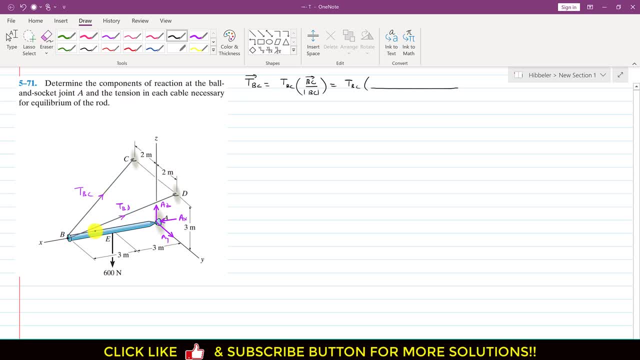 right? So what? this is our unit vector from B to C, right, So to reach this point C we need to travel? how much distance? 3 plus 3, 6 meters in the negative x direction. right, So this B- C vector. 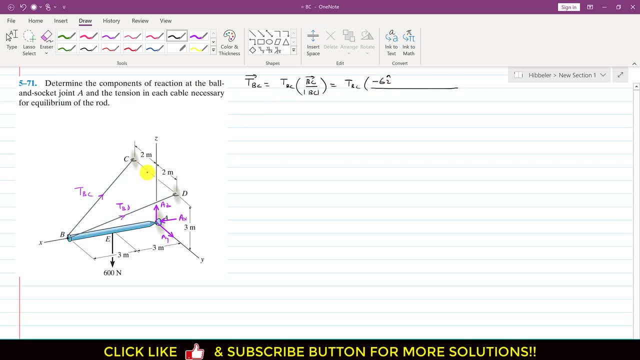 minus 6i, Then we will travel 2 meters in the negative y, So I will write minus 2j, And then 3 meters in the positive z direction to reach this point C right, So we will write plus 3k. 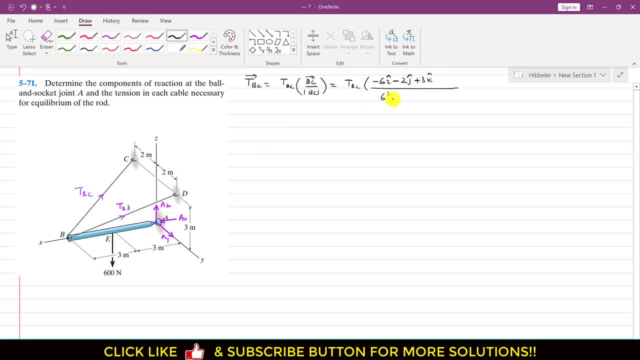 And the magnitude will be minus 6 square plus 2 square plus 3 square right. So this is minus 6 square minus 2 square plus right. So we will take square root. So this magnitude comes out is: this is equal to 7, right, So T B C vector will be equal to minus 6. 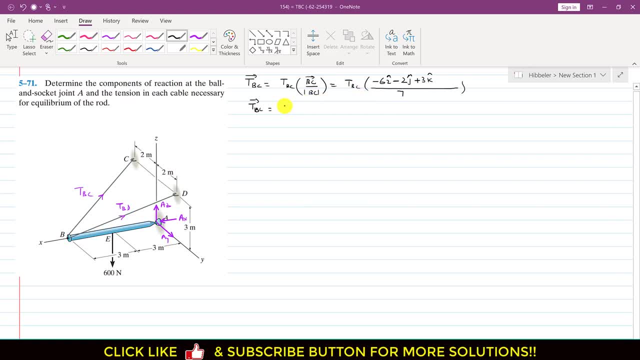 divided by 7, into T B C. So minus 6 divided by 7 T B C, and this is into i, minus 2 divided by 7 T B Cj, And this will be plus 7.. 3 divided by 7 TBCK, And we can write this TBC vector If we simplify this. so then this TBC. 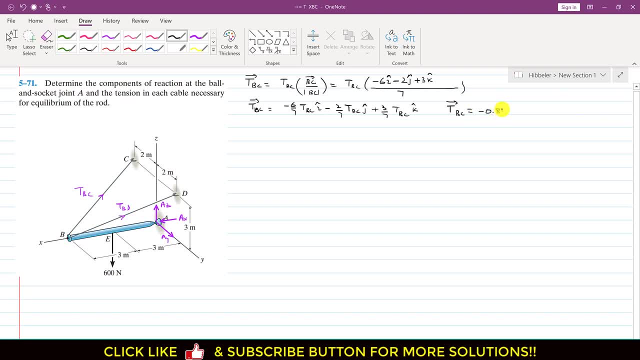 will be minus 0.857 TBCI, minus 0.286 TBCJ, plus 0.429 TBC, and this is along K. Now we can find TBD using the same method, right, But as we can see that this T, this C point, is 2 meters in the Y direction, 2 meters away in the Y direction. 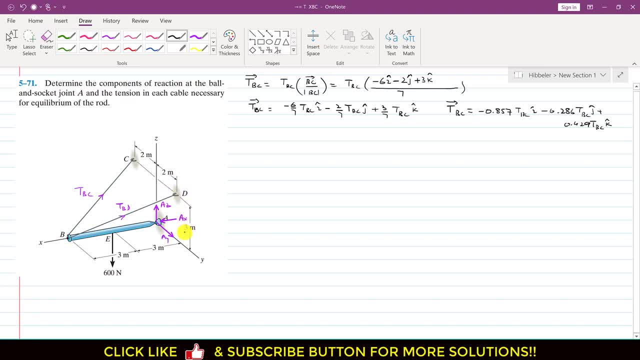 Similarly, this point D is 2 meters away in the Y direction. Similarly, this point D is again at the same height from the Y axis right- this 3 meters- And this point B is at the same location, that is, at the 6 meter right. So what I mean is that this TBD and this TBC. 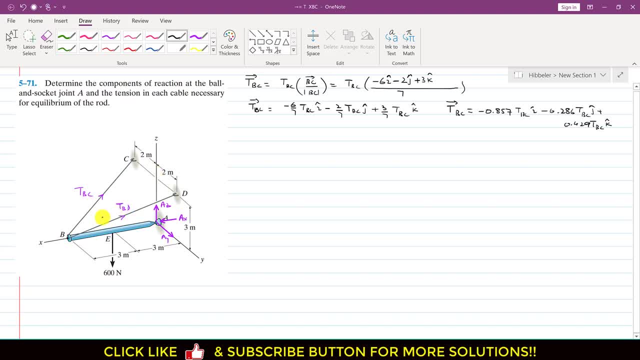 both of these forces are symmetrical about this XZ. So this means that TBD force vector will be equal to this TBC vector, but only this TBD will have one component in the positive Y direction, right. This TBD will have one component in the negative X, and whose magnitude will be the same right. So whose magnitude? 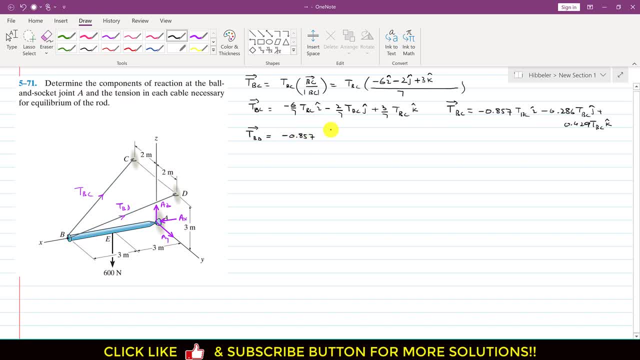 will be minus 0.857 TBCI, minus 0.857 TBCI. Then this TBC, one component of this TBC, was acting in the negative Y. So one component of this TBD is acting in the positive Y, but the magnitude will remain the same since the dimensions. 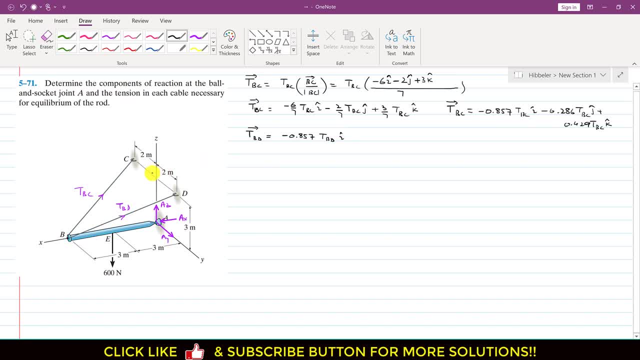 are the same right And the location of C and D points are symmetrical about the Z axis right. So we can write that this will be plus 0.286 TBDJ plus 0.429 TBDJ. So this is our TBD vector. Now the reactions at this point A, if we represent A vector. 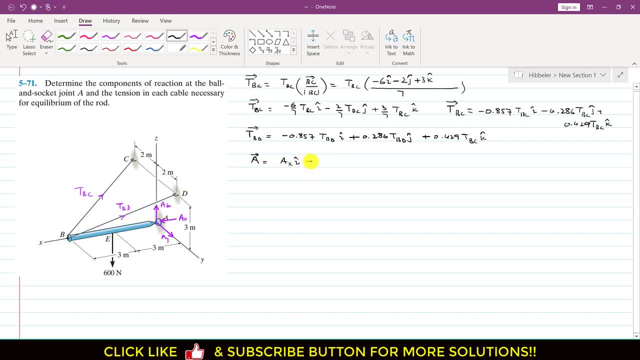 so this will be AXI plus AYJ plus AZK And similarly, if we represent this weight right, this is the weight and this is 60 Newton R. this is some force, right. So let us say that we. 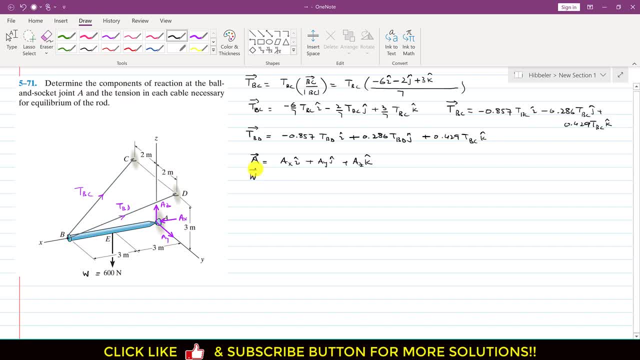 represent that force by W right. So W vector will be equal to minus 600 J, right. Since this 600 is acting in the negative K right. Since this is not J, this is minus 600 K, right. So now in this problem, we are required: 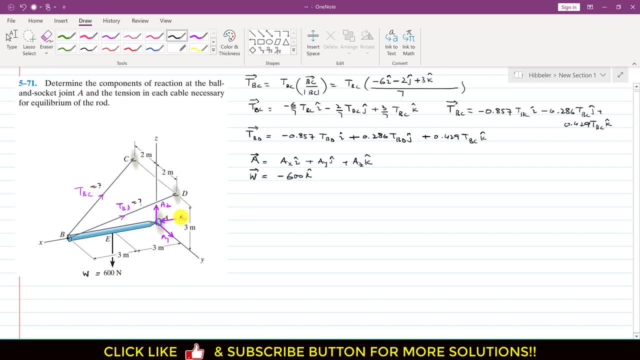 to find this TBC, this TBD and this AX, AY and AZ reactions. right, So, first of all, we will apply the summation of moment at point B equals to 0, right, So, as we can see that this TBD and this TBC. 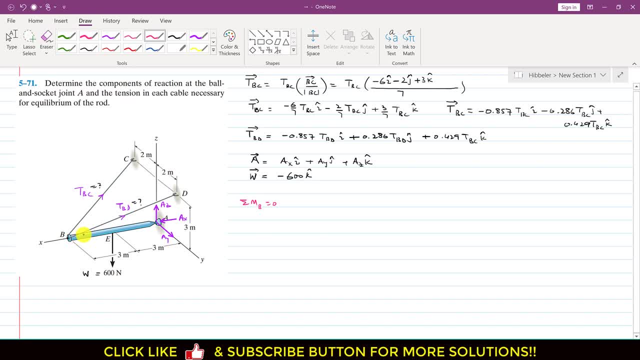 they are intersecting. they are originating from this point B, right, So they will not produce the moment about point B, right? So this means that if we find the moment at point B, so we have eliminated this TBC and TBD and both of these are unknowns right Now, as we can see that. 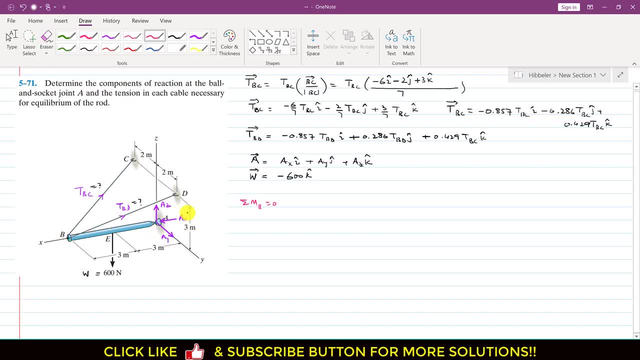 this AX is passing through that point B, so this AX will not produce the moment about point B, right? So we are only left with this AZ, this AY and this 600 Newton force. they are producing the moment about point B. So now we can write that the moment about point B is: if we find 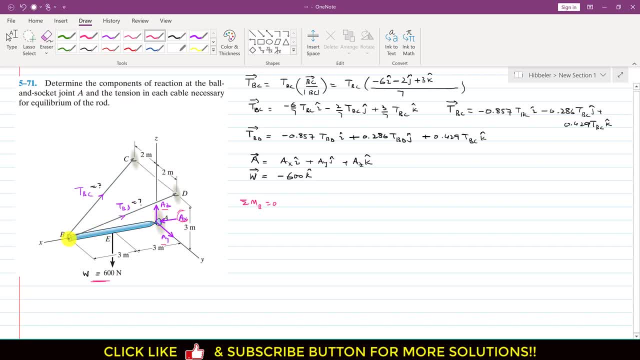 the moment of this AZ. so the moment arm of this AZ will be from this point B to C, right. So this will be the moment arm, right. So this moment arm. if we represent this moment arm as a vector, so then this will be minus 6i. 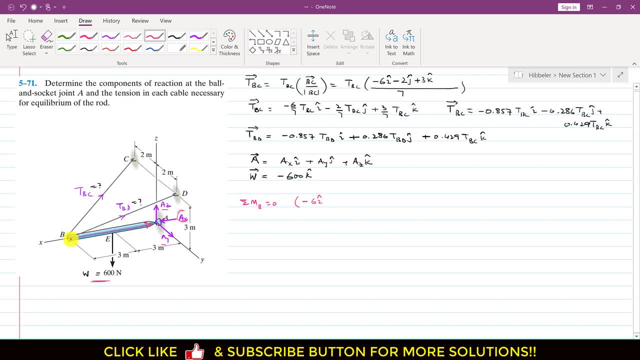 right, since it is acting in the negative x direction and the magnitude of this is 3 plus 3, so this is 6 and this is acting in the negative x. so we will write minus 6i cross and we will write it AZ, and AZ is acting in the positive k direction, right? So this will be the moment. 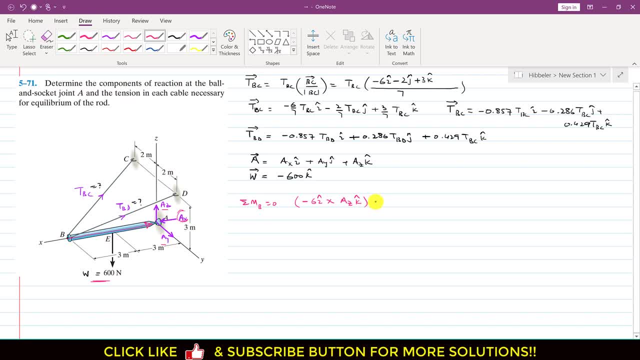 of the AZ component of this reaction, right. Similarly, we will write this moment arm of this AY, we will write plus and as we can see that the moment arm of this AY is the same, this vector right. So again we will write minus 6i, plus AY, and AY is acting in the positive. 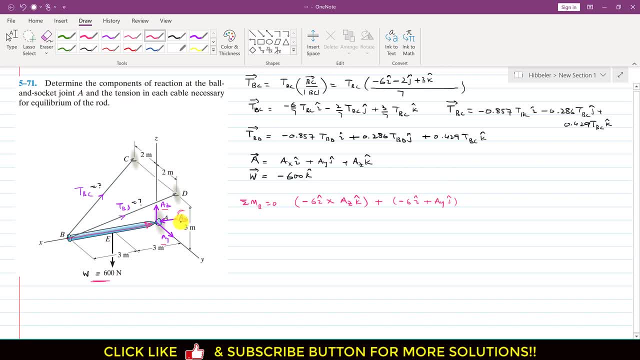 g direction and this AX is not producing the moment, right, So there is no need to write. and now, as we can see that this 600 Newton, this will be plus, and the moment arm of this 600 Newton will be from this point B to E, right, So this is the moment, So this is. 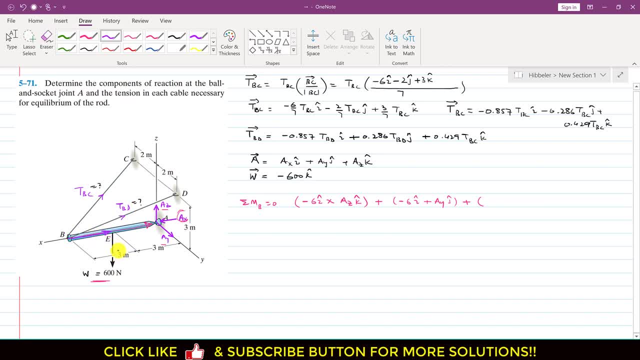 the moment arm right and the magnitude of this moment arm will be how much? So this is 3 meters right and this is going to be minus 3, since we are going in the negative x direction. So we will write minus 3i and cross. sorry, this is cross, right, Remember. 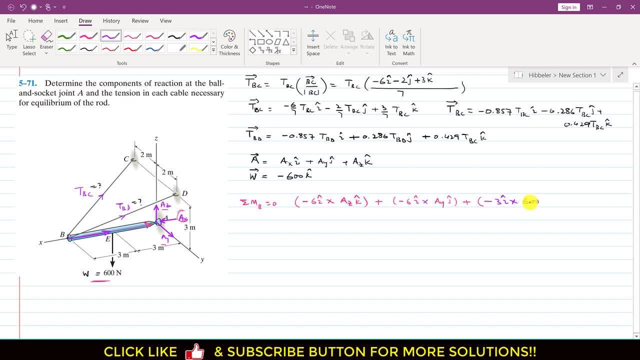 this is cross cross 600 and this 600 is acting in the negative k, So we will write minus 600 k. Now let me draw this: i, j and k right. So now, if we apply this cross product, so this will be minus 6AZ and. 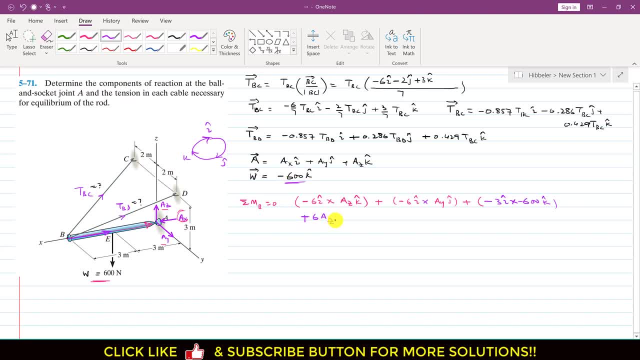 i cross k, So i cross k is minus j, So this will become plus j. Similarly, it will be plus minus 6AY and i cross j, So i cross j, is k right? So this is minus 6AZ. 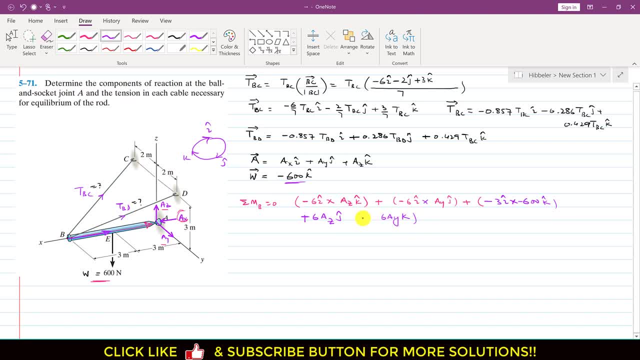 So minus 6AYk, or we can write it directly as minus 6AYk. Similarly, if we multiply this so this will be plus 3 into 600.. So this is 1800 and i cross k. So i cross k is again. 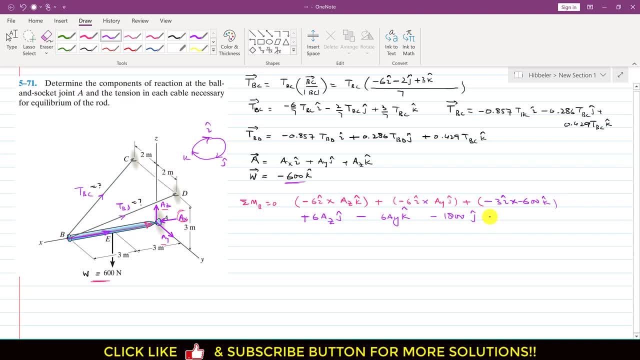 minus j. So we will write minus j, and this will be equal to 0.. Now, as we can see that both of these are j terms, right? So we can write it like this. So this will be 6AZ minus 1800, j minus 6AYk, and this will be equal to 0,. 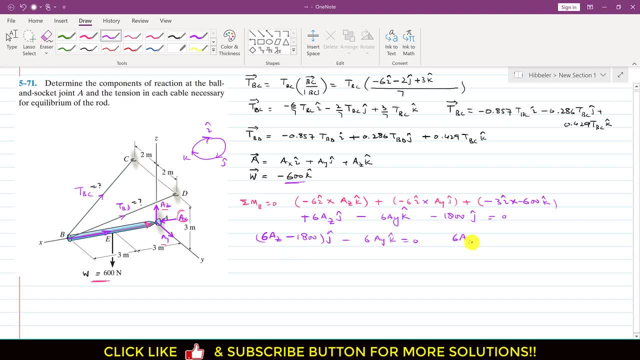 right. So this means that we can write it like this: So 6AZ minus 1800, this component will be equal to 0 and minus 6AY will be equal to 0.. So from this we can conclude that 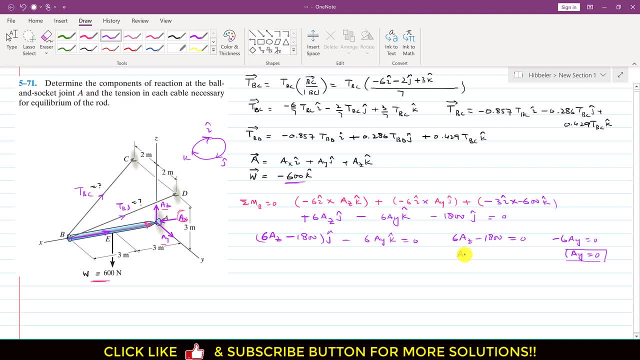 AY reaction is equal to 0. And from this we can say that is equal to 300 newtons. So now Az is known, this is 300, Ay is known, this is 0, so we can remove it. So now we are left with both of these reactions, and Ax is unknown and Az. 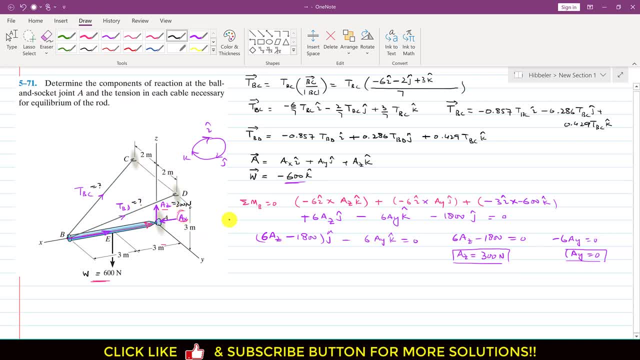 is known. So now if we apply the summation of forces along x equals to 0, let us say, if we apply the summation of forces along y equals to 0. So now we have these force vectors. So along y we have this 0 point. we can write that this will be minus 0.286. 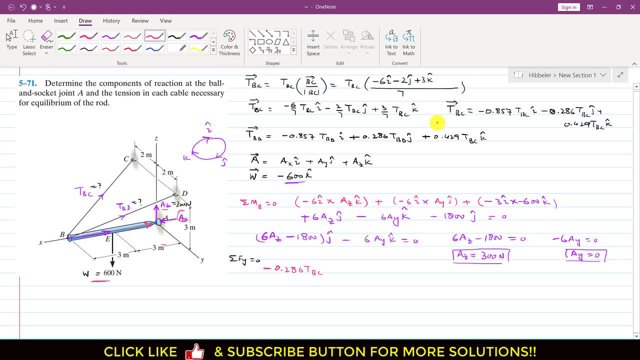 Tbc, the component of Tbc acting in the y direction, plus the component of Tbd acting in the y direction. So this will be plus 0.286 Tbd plus 0.286 Tbc acting in the y direction. So this will be equal to 0, and since we know from this that Ay equals to 0.. So this is: 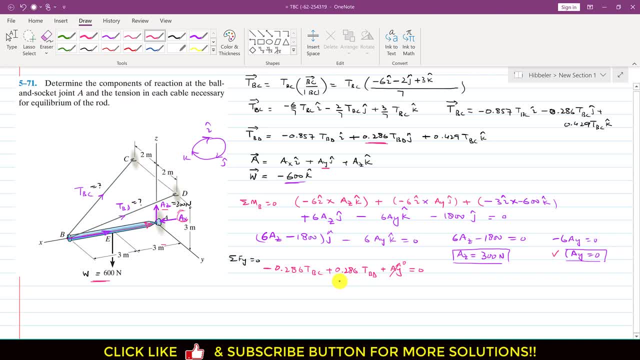 equal to 0. So from this we can say that Tbc equals to Tbd. This is very important reason. So Tbc is equal to Tbd. Now if we apply the summation of forces along x summation: 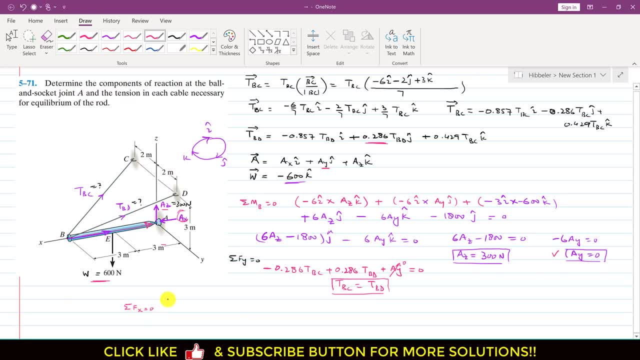 of forces along x equals to 0.. So we will add up all the components of the forces in the x direction. So now, as we can see that this is minus 0.857, minus 0.857 Tbc, This is acting in the y direction. Similarly, this minus 0.857 Tbd, and this plus Axi, So plus. 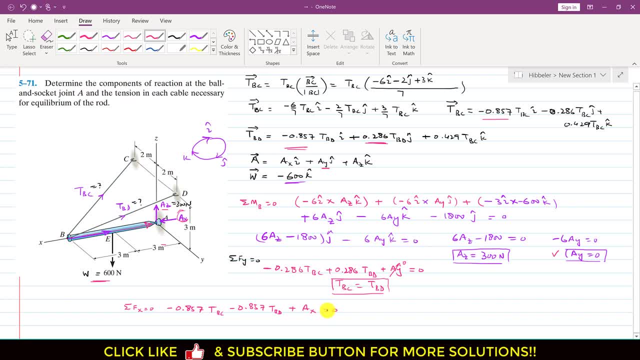 Axi, And this will be equal to 0.. So, from this conclusion, we can write Tbd as Tbc, So we can replace this by Tbc, since both are equal. So this means that if we add up both of these, 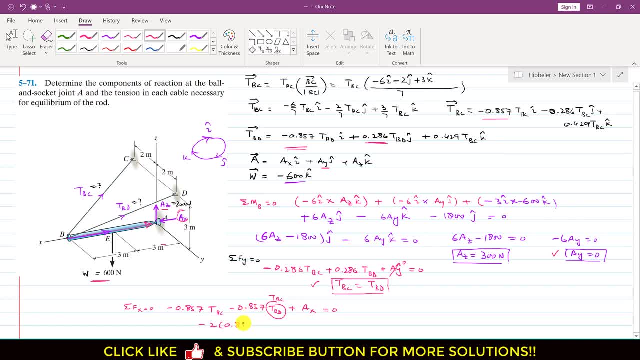 so this will be minus 2 into 0.857 Tbc and this will be equal to minus Ax. So let us say that this is equation 1.. In this equation, Tbc magnitude is not known And the x magnitude is not known, Right? So we have only Az magnitude and Ay magnitude. 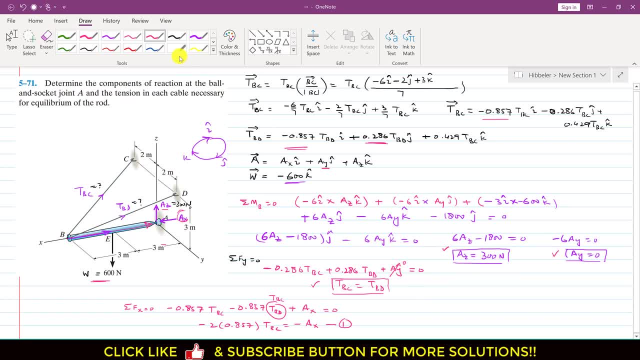 right. So now this means that we need one another equation. So let us say that if we find the summation of forces along z equals to 0.. So now we have to add up all the z components of the forces, right? So this will be 0.429.. So this will be 0.429 Tbc. This is plus 1.240 Tbc, So this is equal to Tbc. So this is equal to 0.429 Tbc. So this is equal to 0.429 Tbc entitled to 0.420 Tbc. So now we can write down. so this is: 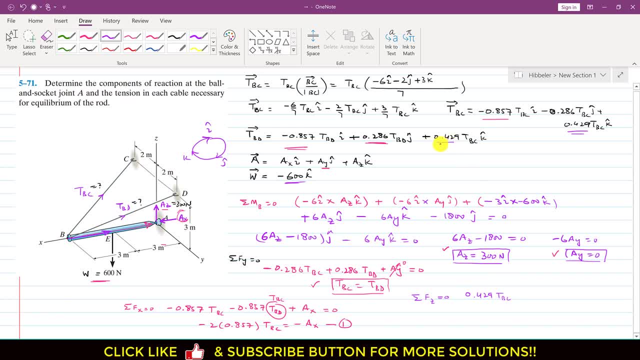 0.420 Tbc. So this is equal to 0.420 Tbc. So this will be 0.420 Tbc, So this is equal, is plus 0.429 Tb. this is Tbd. remember this is Tbd, So we can write Tbd as Tbc. So this: 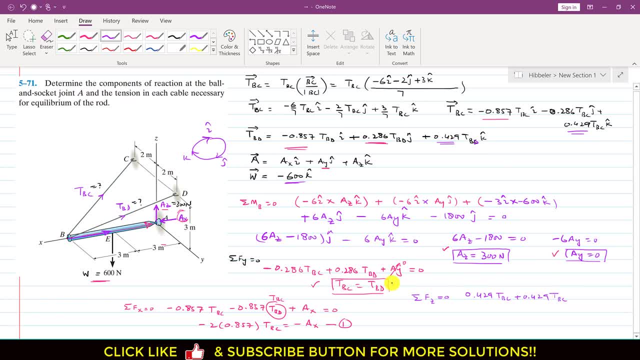 is Tbc, since Tbc and Tbd are equal, and this will be plus azk. So this is az and this is also acting in z direction. So this will be minus 600 and this will be equal to 0.. So now we know az. So this will become 2 into 0.429 Tbc and this az is 300.. So 300. 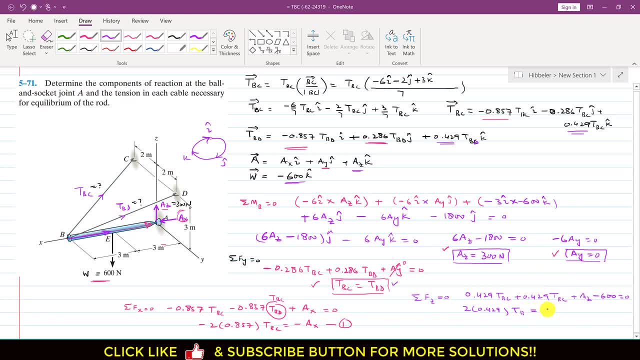 minus 600 is minus 300 and on the other side of the equation, So this will become plus 300. So this is Tbc. So Tbc will be 300, divided by that thing, and 3 Tbc comes out to be 350 Newtons. So this means that Tbc, which is 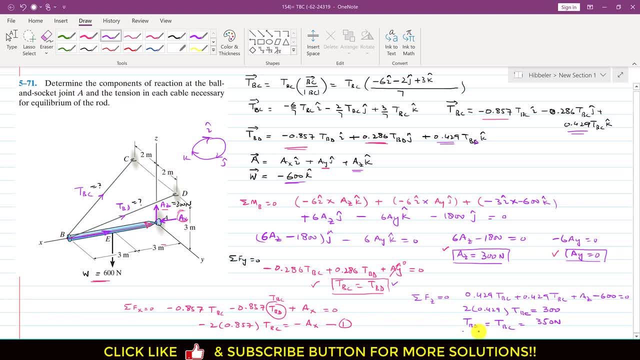 equal to Tbd is equal to 350 Newtons. So now, since we know this Tbc, so we can incorporate this Tbc in this equation 1.. So this will give us ax. this minus sign will cancel out. So this means that ax reaction. 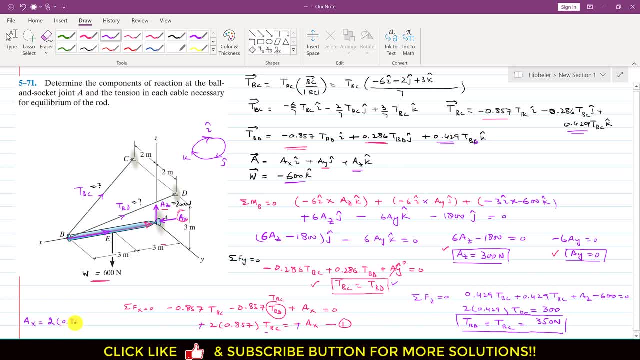 ax is equal to 2 into 0.857, into 350.. So from this ax equals to 600 Newton. So now we can say that ax is equal to 600 Newton, ay is equal to 0,. az is equal to 300 Newton. 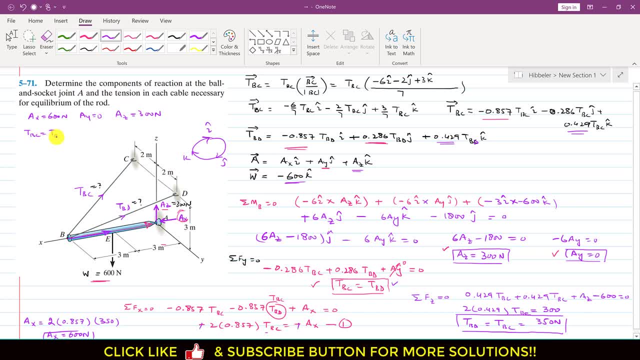 And Tbc equals to Tbd equals to 350 Newton. So this is the solution of this particular problem.